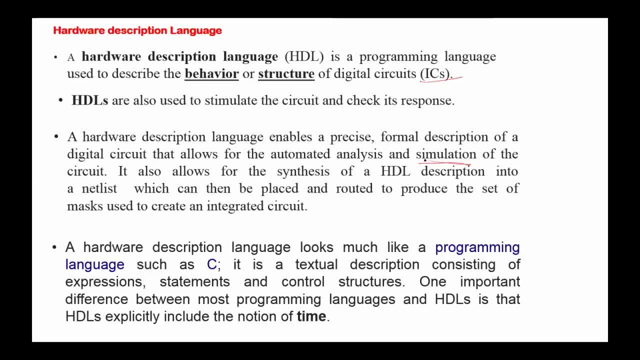 It also allows for the synthesis of a HDL description into a netlist, which can then be placed and routed to produce the set of masks used to create an integrated circuit. A hardware description language looks much, Much like a programming language such as C. 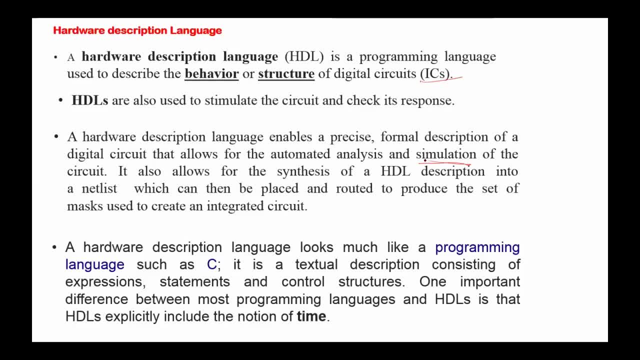 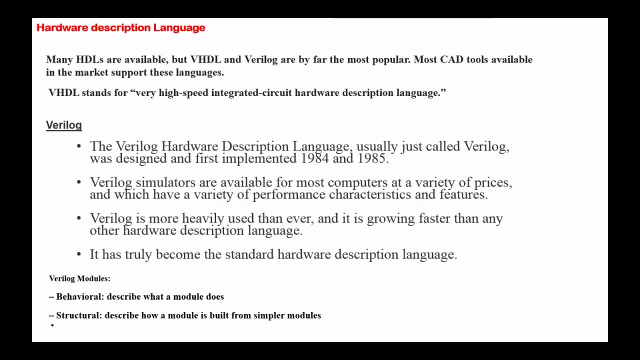 It is a textual description consisting of expressions, statements and control structures. There is one difference between HDLs and programming languages in that HDLs explicitly include the notion of time. There are several hardware description languages available, but the most common used are VHDL and Verilog. 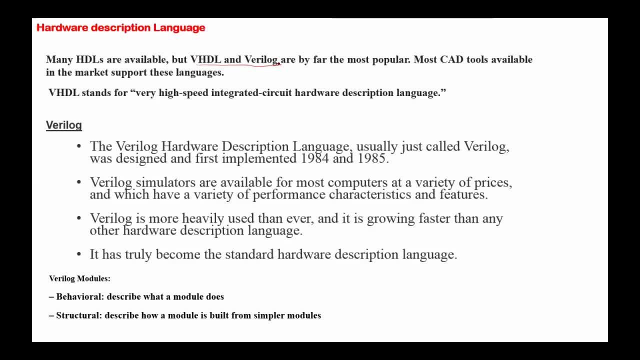 VHDL stands for. VHDL stands for Very High-Speed Integrated Circuit Hardware Description Language, where Verilog is from verifying logic. Verilog was developed by IEEE and has become the standard hardware description language and there are several versions of it: in 2001 and a version in 2005.. 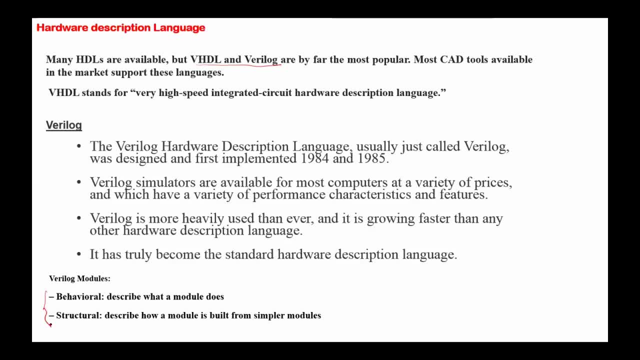 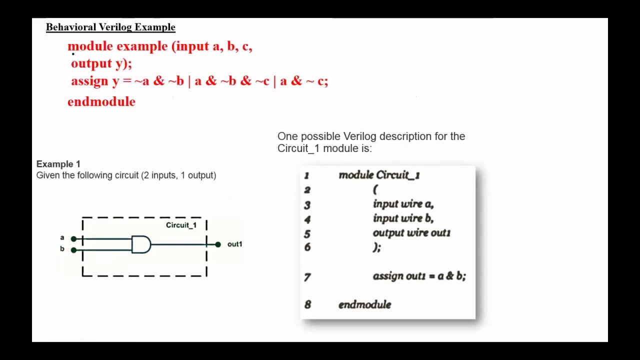 Verilog modules are of two types: behavior and structural Behavior describes what a module does, While structural describes how a module is built from other modules. Here is the behavior Verilog example. The words module and endmodule are reserved, assigned as well. 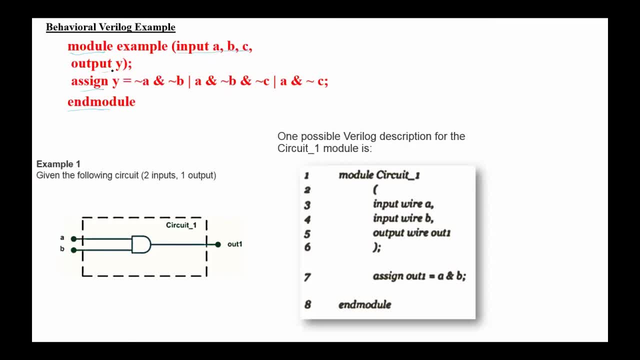 Here we have the inputs, the outputs and the outputs, And the output is assigned the logical expression. Here is one possible description for the AND gate using Verilog: we have inputs a, b and output one. here in the module we have input wire a. 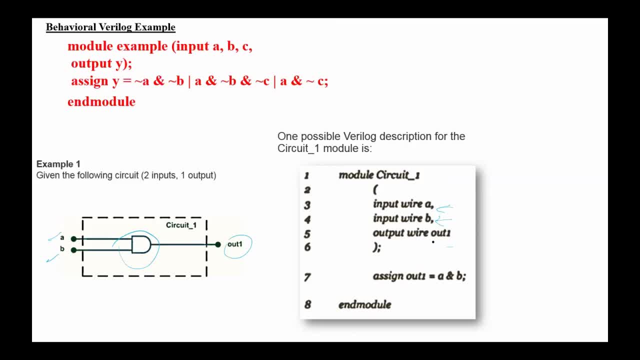 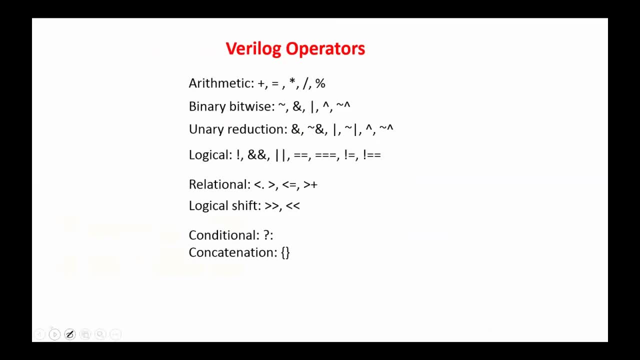 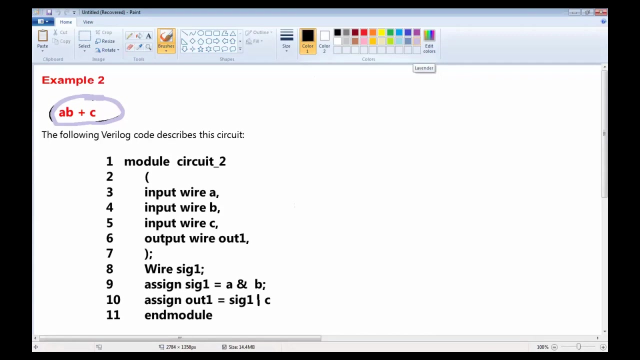 input wire b, output wire one, and we assign the outwear a and b. these are the most common used operators in hdl languages. here are the blog operators. they are similar to the symbols used in programming languages and in mathematics. here we have another example: the expression a, b or c, the 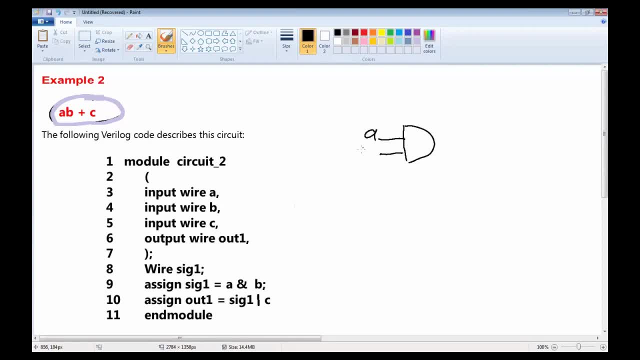 circuit is as follows: a, b, c. in the description we have the input wire a, input wire b, input wire c and we have the output wire out. one wire signal one is defined here and sig one is assigned a and b and the output is assigned sig one or this is the operator for, or operation or c. 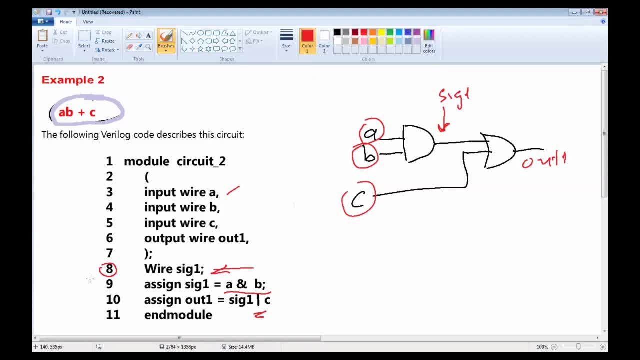 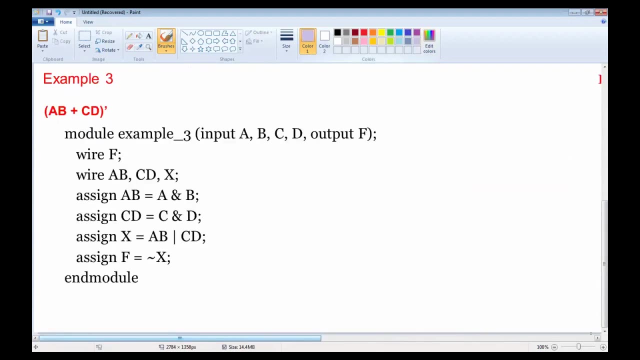 as you see in line 8, an internal signal is defined. the keyword where is used to specify the data type of this connection. the wire data type would translate to a physical wire in the design. here we have another example: the expression a, b or cd or not. 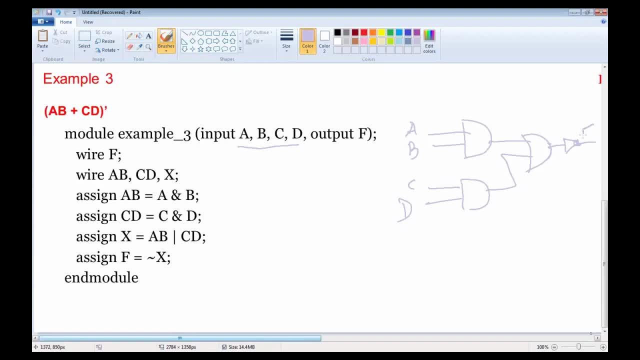 inputs are defined. abcd. output is defined as f here. here we have the wire a, b and here the wire cd and here the yx. the wires a, b, c, d and x are cleared. we assign the operation a and b to the wire a b, the operation c and d to the wire cd and the abrir还是. 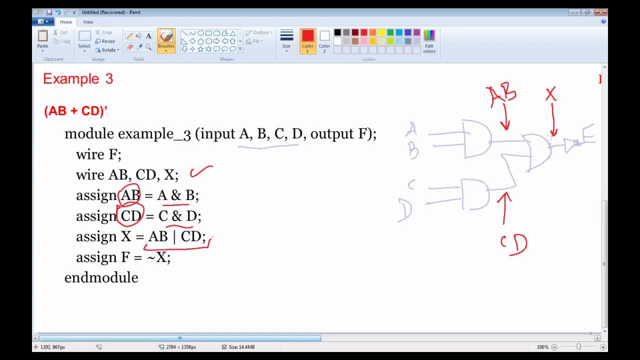 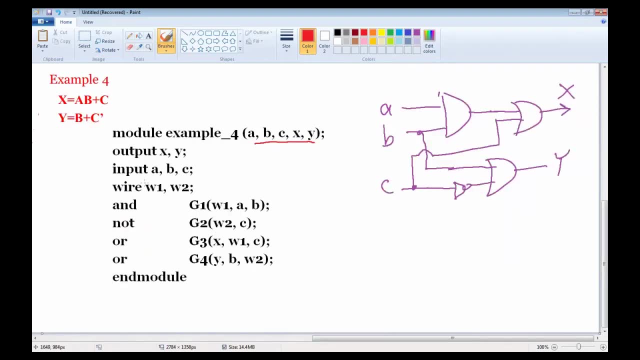 from these two wires is assigned to the wire X and finally, not X, is assigned to the function F. Here is another example with two functions: A, B, C are declared as inputs, X, Y as outputs. Now we have two wires, wire one and two are declared. 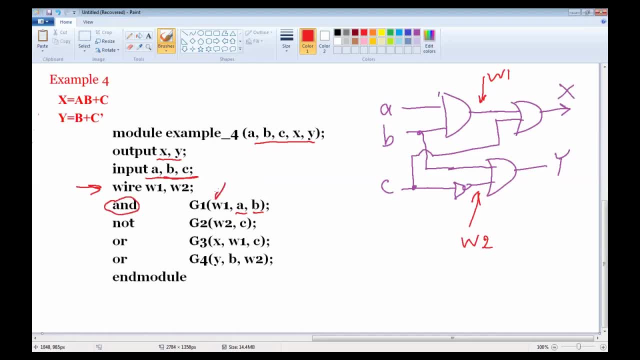 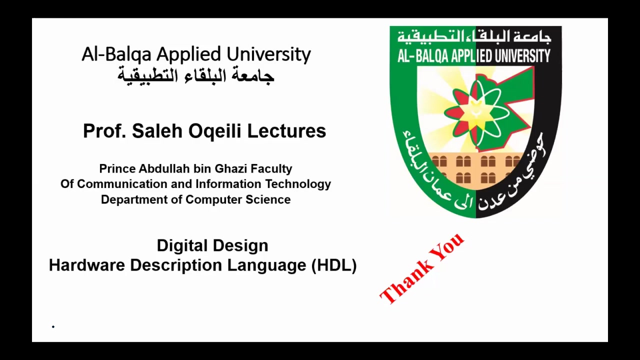 Next we add A and B to wire one, We complement C into wire two, We add C or wire one into X and we add B with wire two into Y. This was a quick introduction to HDL. This introduction is good for computer science students. 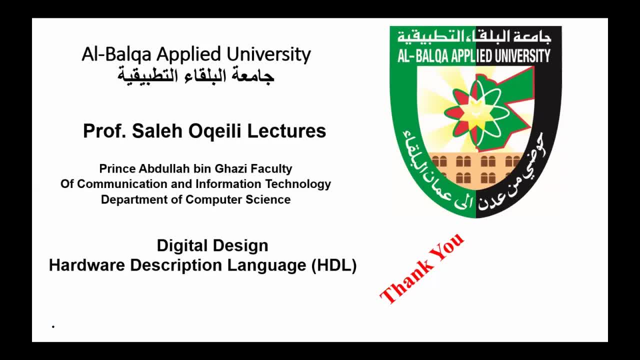 However, engineering students need to exercise and learn more in order to use HDL simulators. Thank you, Thank you.